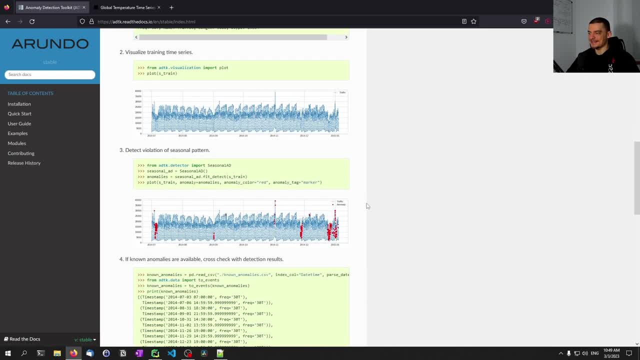 then we plot the sequence or the series and then we use a detector. in this case, they use the seasonal detector to find anomalies, and what detector you use depends on the use case, but anomaly detection can be very useful for a bunch of different tasks. so, for example, one thing that comes to mind is you. 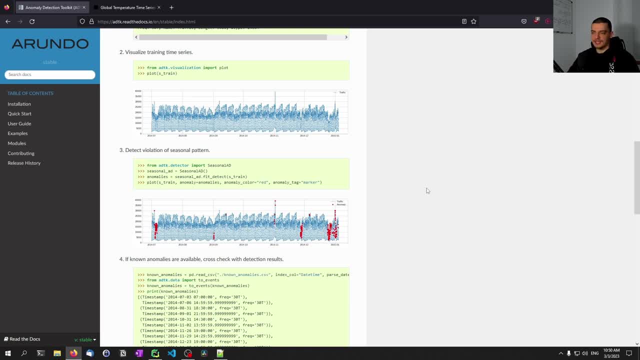 might have a server. a lot of users are connecting to that server and you keep track of some measure, some metric that is related to user activity, on a minute-to-minute basis, for example, and when you find an anomaly there, when you detect an anomaly, this might be assigned for an attack, or maybe you 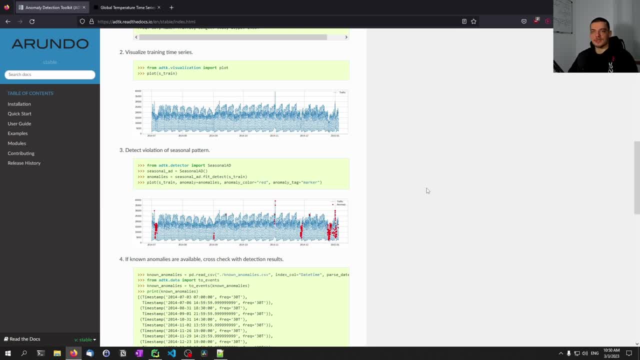 just get more traffic because someone mentioned you. but maybe you want to be notified when something unusual happens because it might indicate an attack, and then you might want to set up an attack and take certain measures. also in stock data you might want to spot some anormal data, some 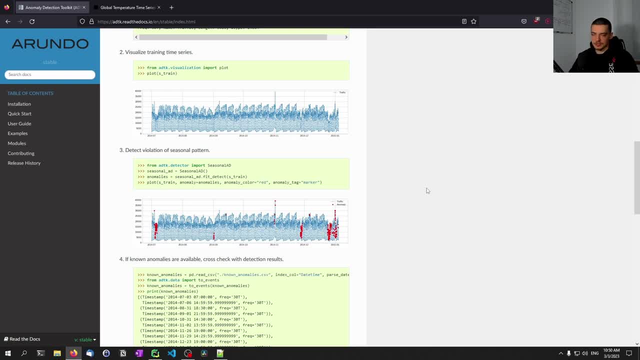 anomalies in price movements. maybe a lot of selling is going on, a lot of buying is going on, the volatility is very unusual, or the volume is very high, the volume is very low, something like that. this might also help to inform, to make informed buying or selling decisions. so this is what we're. 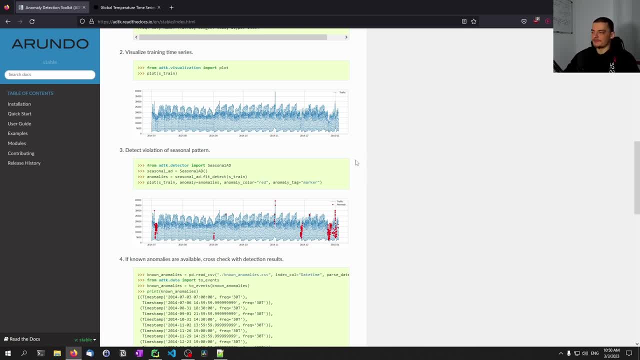 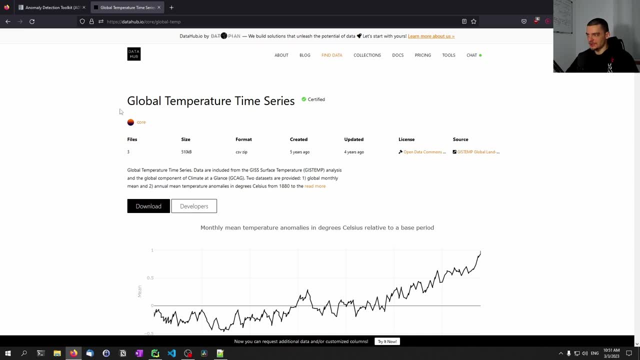 going to talk about in this video. we're going to talk about this toolkit and for this we're going to have to use time series data. i'm going to use two different data sets. one is going to be the temperature- global temperature, time series data set here. 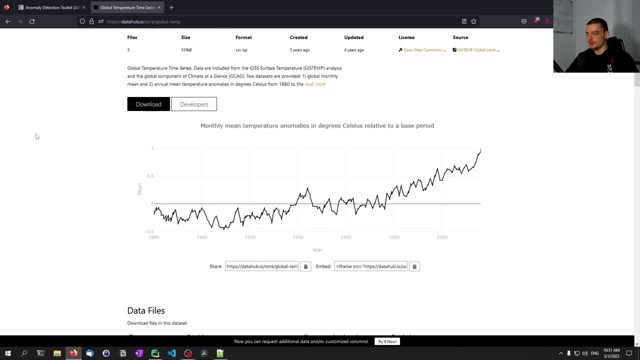 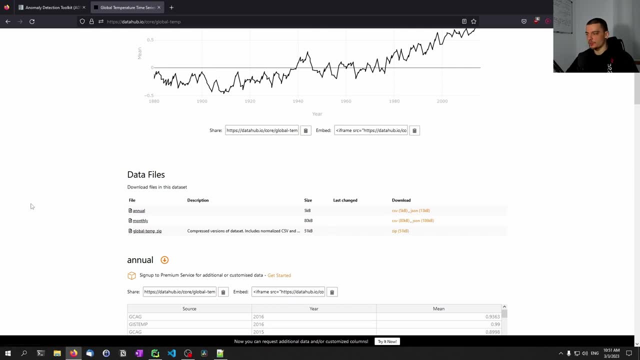 from data hub io. you will find a link in the description down below. basically, you just have to download here this monthly data as a csv file and store it in the directory that you're going to be working in. and in addition to that, i'm also going to use stock data, maybe of multiple 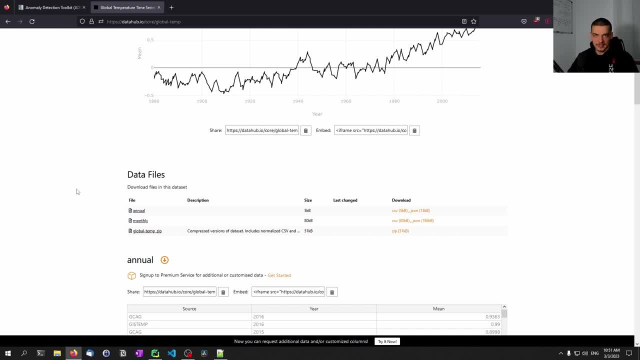 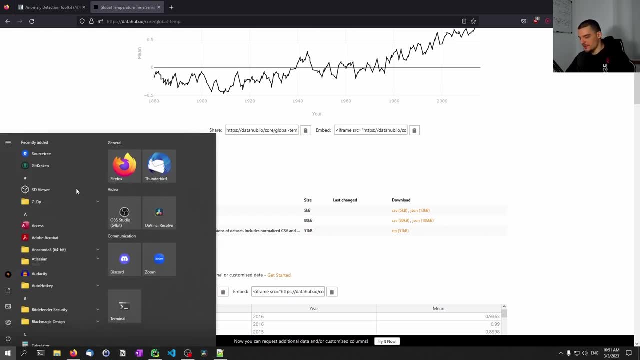 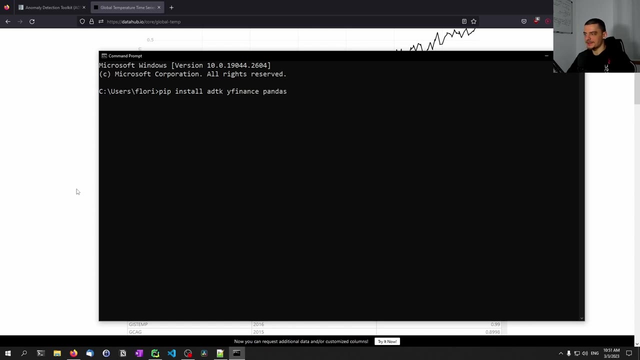 different companies, and for that we're going to use the y finance library, which allows us to access the yahoo finance api from python. so the first thing we want to do is want to open up the command line and we want to type pip, install adtk, y finance, pandas and matplotlib. those are going to be the libraries. uh, those are the. 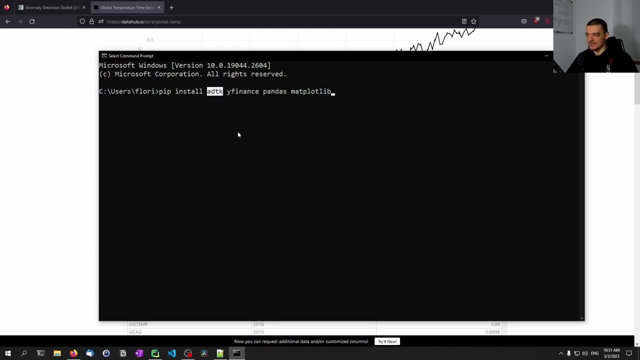 libraries that we're going to be using: the advanced, not the advanced- the anomaly detection toolkit, the y finance uh library, pandas for loading the data set and matplotlib for displaying the visualizations. so install these packages and then we can get into the code we're going to start. 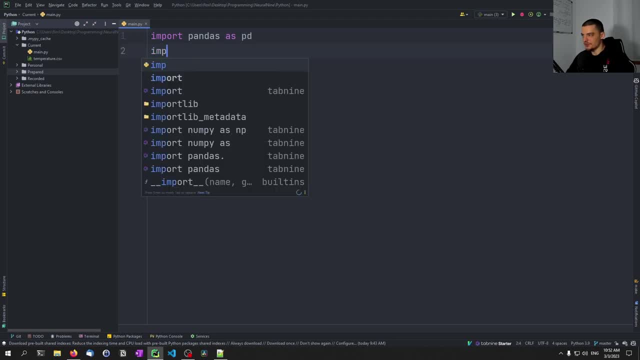 with import. we're going to import pandas, spd, we're going to import matplotlib, dot, piplot, splt. we're going to import y, finance, syf, and then we're going to import from adtk dot data, the validate series function. then we're going to say from adtk. 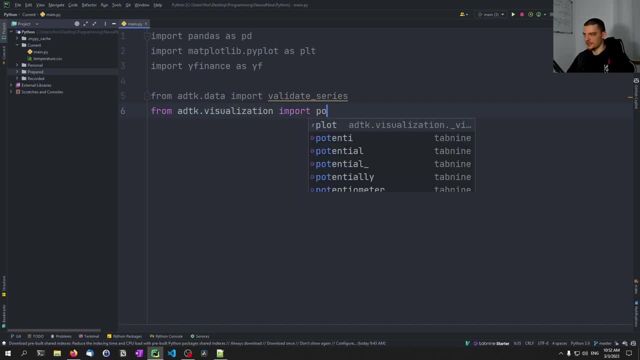 dot visualization. we're going to import the plot function, say from adtk dot detector, and in this case, here, for the sake of simplicity, i'm going to use a wild card import. uh, this is, as always, not a good practice, so you should always um explicitly import things like threshold ad, seasonal ad, quantile ad and so on. but since we're going to 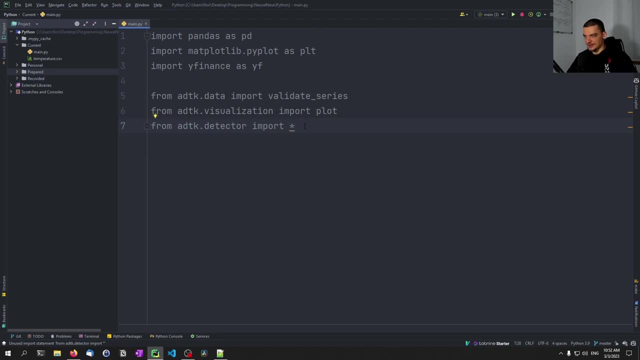 use so many in this video. today i'm just going to use, uh, this wild card import here, so basically import everything, all right. so let's get started by loading the data set first. i already have this temperature csv data set here on the left in this directory and we're going to start by saying: 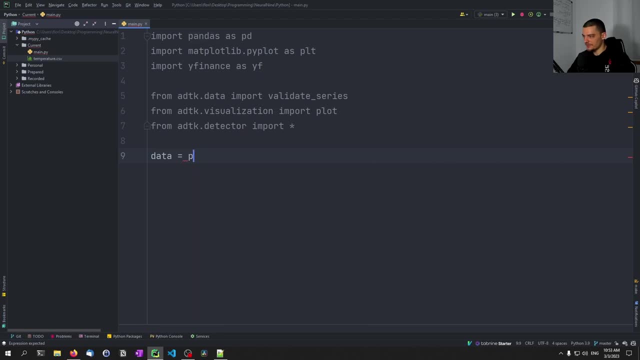 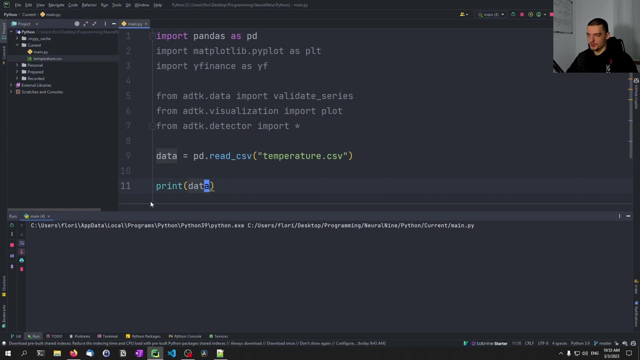 the data is going to be pd, read csv, temperature csv. we can print that to see if that works. and what's important here is we need to have a certain structure, we need to have one feature and we need to have the date- a date time, um instance- as the index. so in this case, 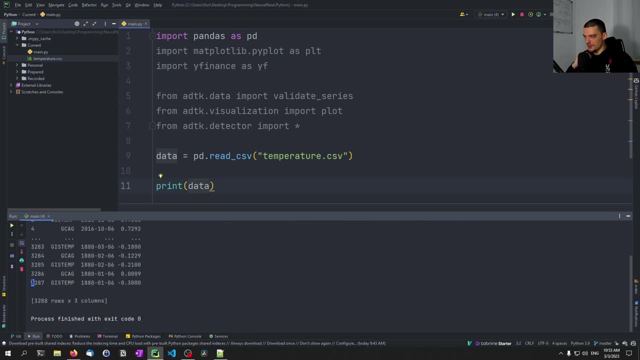 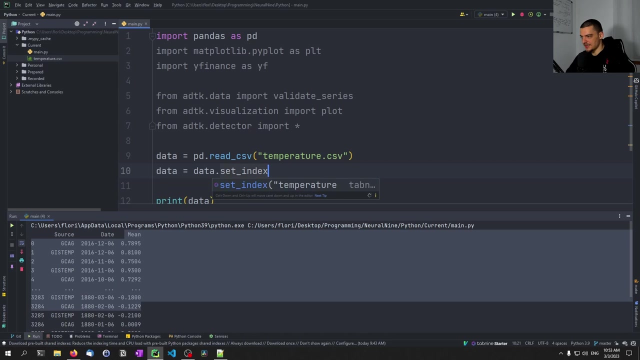 we have, uh, just a basic index from zero to 3287. uh, we need to drop the source column, we need to to make the date column the index and we need to keep the mean column. so what we're going to do here is we're going to say data equals data, dot set index date, and then data equals data. 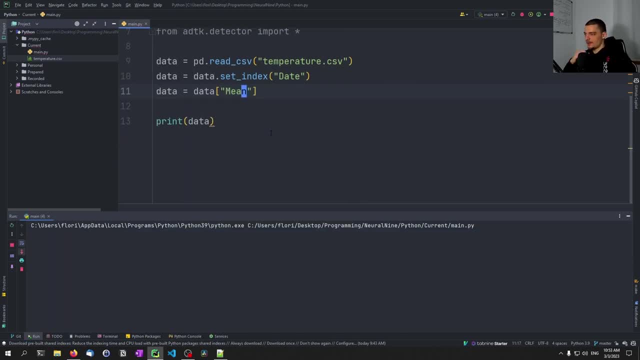 mean like this: and this results in the data set index. ok, so we have our standard value. for quick Spelling, for example, fixed decrease indicator will provide us as much of the range we need to be able to reduce as much of the value as possible. now, if we switch to our analog object here, you can see that we have our old delta set. 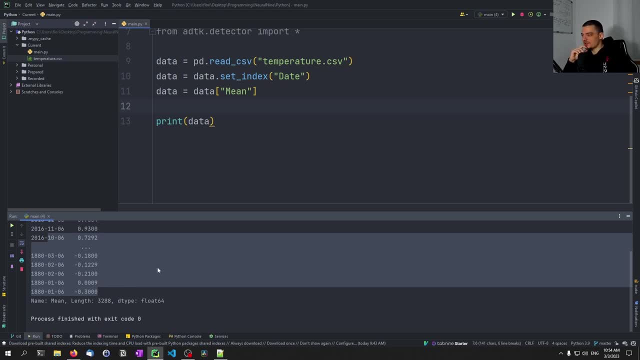 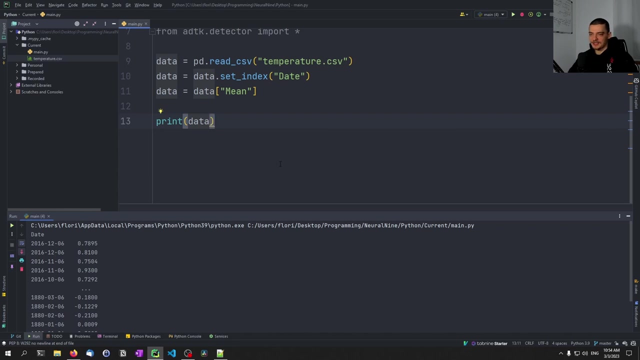 values now. ここはベースです, so we can leave as much value as possible. top cd value, so we can focus wherever come grow, aquí aussi. anomaly detection. and we're going to start with a very basic anomaly detection first, which is going to be the threshold detection. so the threshold detection is quite simple, we just provide. 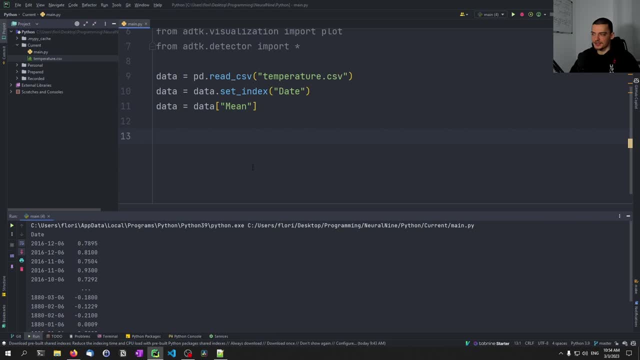 manually a threshold, a minimum and a maximum, a high and a low or a low and high, where we say: okay, if it's below that value it's an anomaly, if it's above that value it's an anomaly, and then we just define anomalies like that or we detect anomalies like that. this is very simple. we can do that. the 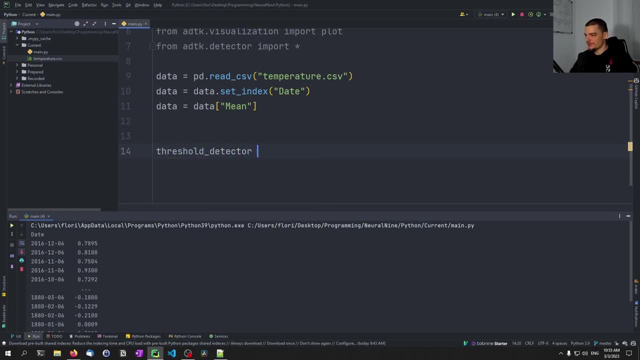 following way. we just say threshold detector is going to be equal to threshold ad low equals. for example, for this data set it makes sense to use something like negative 0.5 and a high is 0.75, for example. then, in order to get the anomalies, we say anomalies. 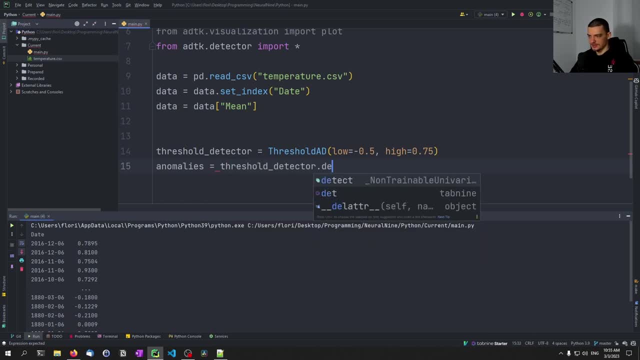 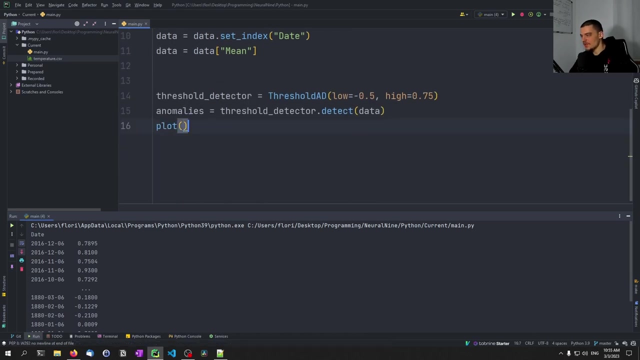 equals threshold detector, dot detect, and then we use the data here. so and then we can plot this very easily. now, keep in mind: this plot function is not mathlibplot, it's adtk visualizationplot. so we're going to plot here now the data we're. 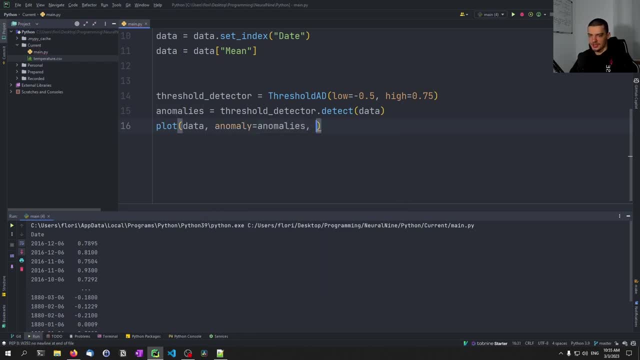 going to set anomaly equal to anomalies. we're going to say: anomaly color equals red and we're going to say anomaly tag is going to be marker and then we just say: plt, show to display the actual results. and that is a very basic anomaly detection we just define. 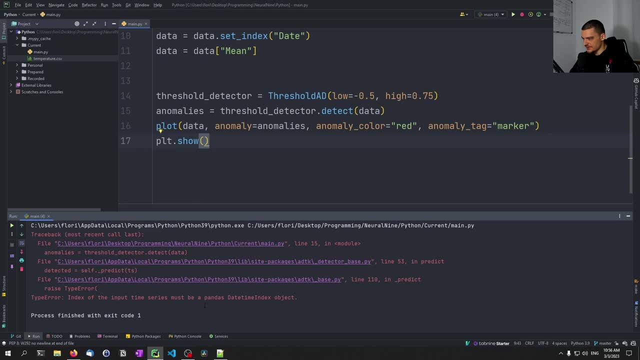 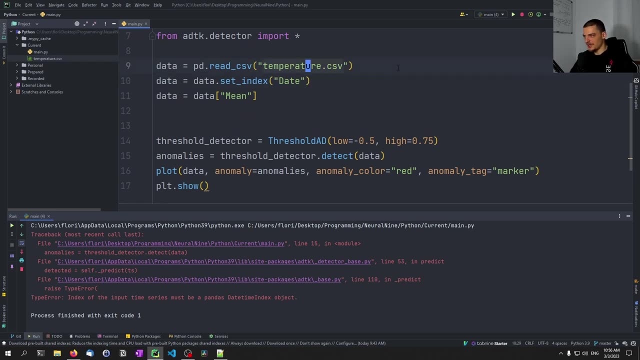 what's the problem here? index of the input time series must be a pandas daytime index object. i think the problem is that it is not by default, maybe it's a string. so what we're going to do here is we're going to say data date is equal to pd. 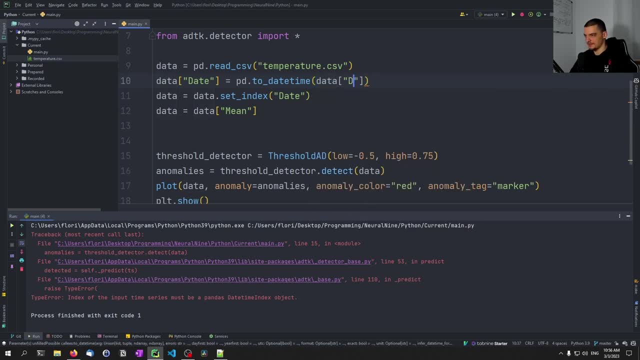 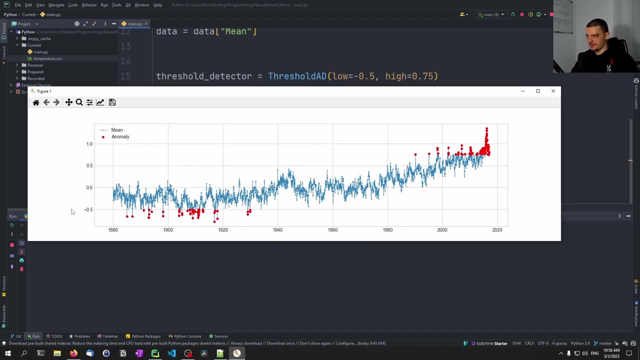 to daytime data date. that should fix the problem, and and and it does so. here you can see now how this works: our low is here at negative 0.5, our high is here at 0.75, and everything above that high or below that low is considered to be an anomaly. 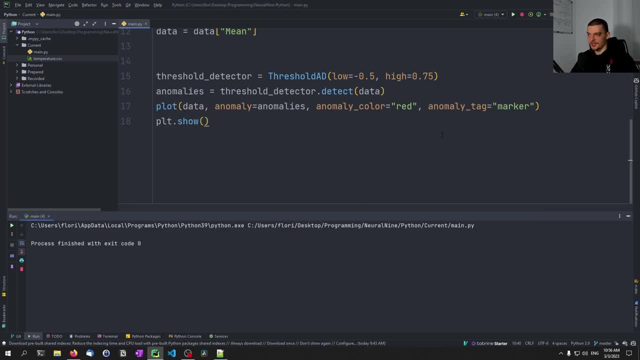 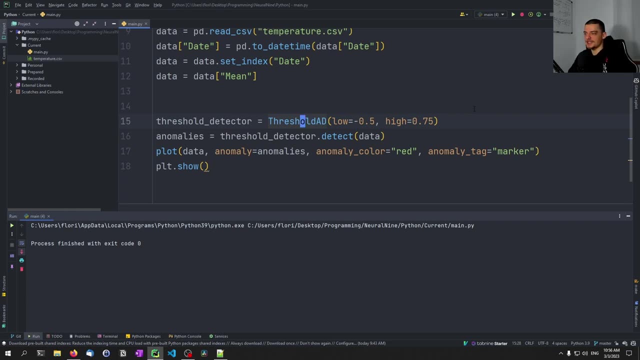 that's quite simple. there's not much much intelligence involved here. we can do something similar with quanta. so instead of providing absolute values, we can provide quanta. so we can say if it's in the 99th percentile, or if it's in the 0.01 percentile we can say it's an anomaly. 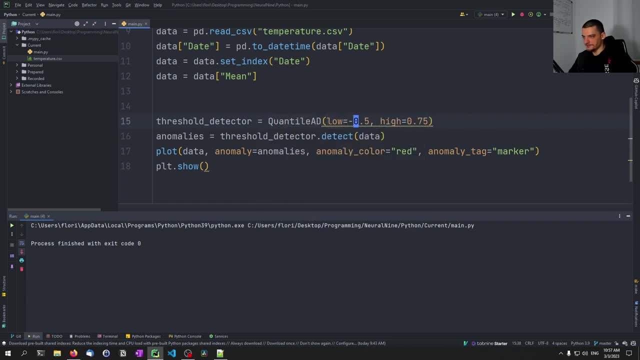 and we do that by saying it's a quantile ad and instead of providing high and low- or actually we do still provide high and low, but we provide them as quanta. so 0.01 or high is going to be 0.99 and we can change the name here also to: 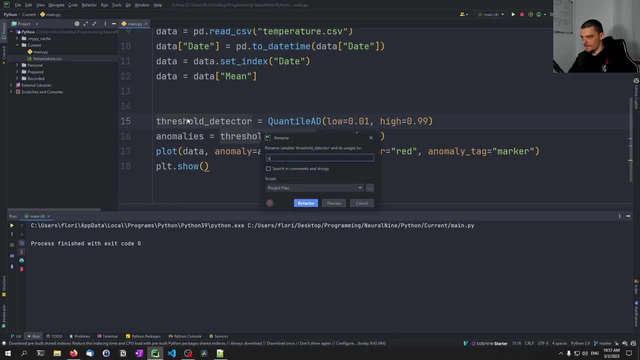 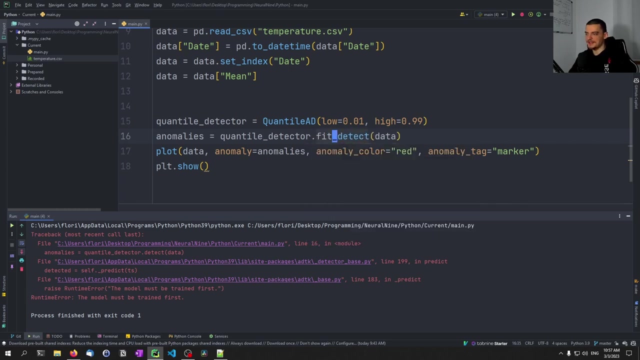 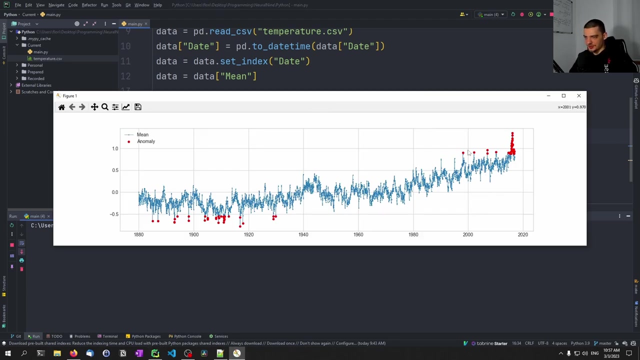 0.99 quantile detector. there you go. let's run this here. and in this case, model must be trained first. yeah, if we use the quantile detection, we need to say fit detect, because we need to train it first on the data, and in this case we can see here all these values are. 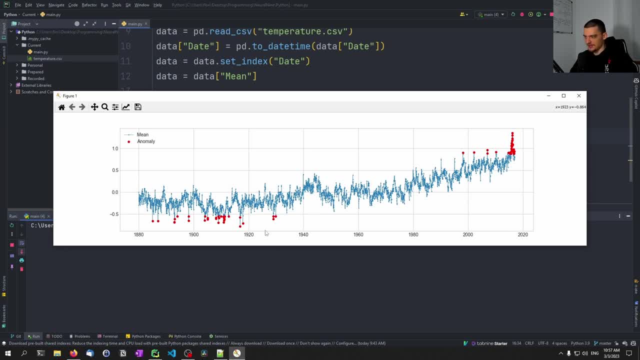 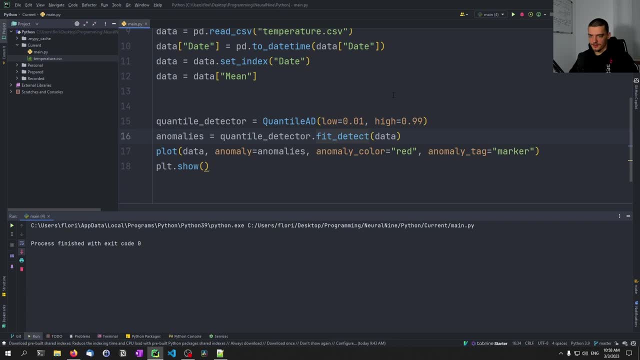 in the 99th percentile. all these values here are in the in the first percentile and those are considered to be anomalies. this is another method we can use, uh. one more method we can use is we can use the interquartile range, anomaly detection, basically meaning we have this uh interquantile. 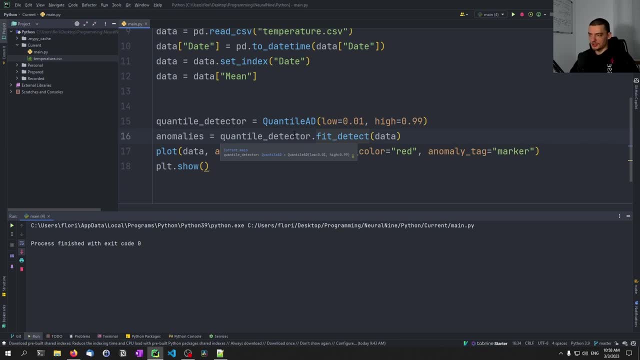 range iqr and we can use a multiplier to say, okay, we allow for that many ranges until we consider something anomaly, so that much deviation from the mean is allowed and other than that all of the other values are considered anomalies. so we can say here: iqr detector is equal to interquartile range. 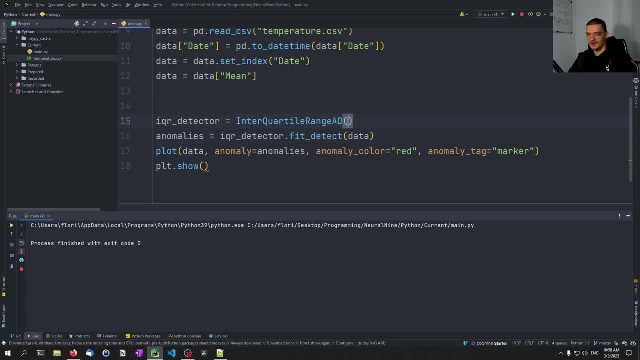 ad, and here we don't provide low and high, we just provide c, which means 1.5 iqrs are allowed. the higher we set that number um, the less anomalies we're going to find. so in this case here we find only those if i set this number to. 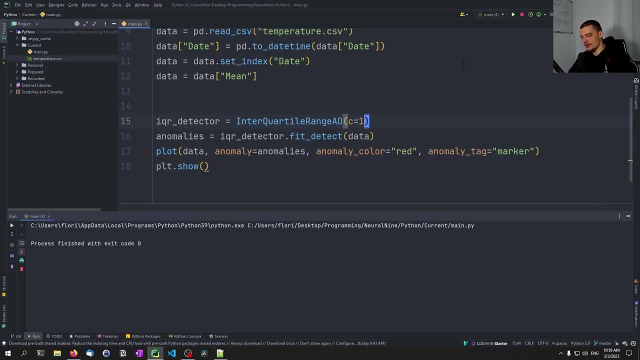 one, we should be able to find the number of anomalies that we're going to find more, because we only allow for one iqr. there you go, we find more of them. if i set this to two, we're going to find less. that's the idea behind this one. um, also, we can use a so-called generalized extreme, studentized. 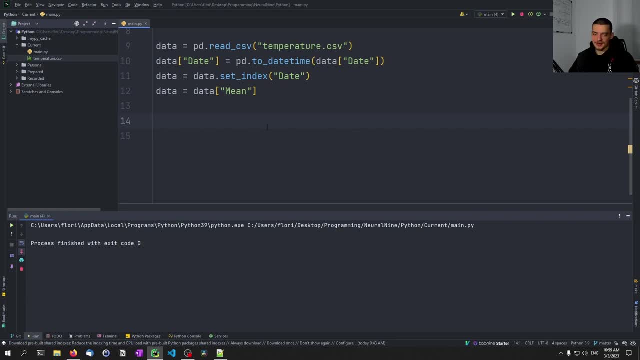 deviate uh test, which is esd. i don't know exactly how it works, don't ask me, but basically what you need to know about this detector is uh. it assumes a normal distribution, so you should only use this if the data actually is normally distributed, or at least if the assumption that the data is 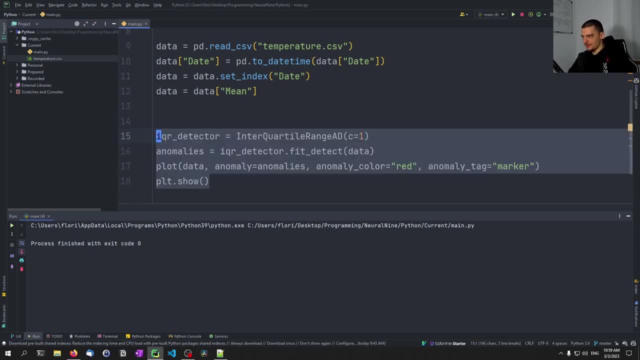 normally distributed makes sense. um, so let me just reverse this: here we're going to say esd detector and we're going to say here generalized esd test ad, and what we provide here is a parameter alpha. let's set it, for example, to 0.3 and, as i said, this is assuming that the data is normally. 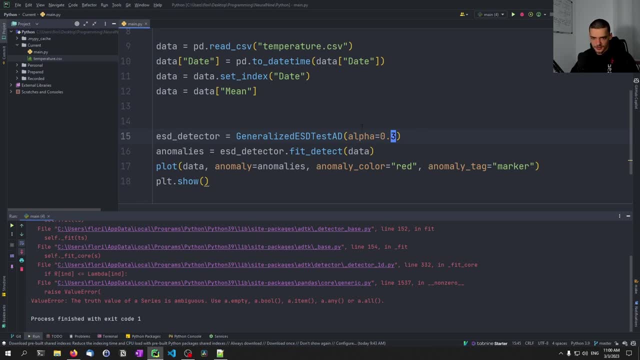 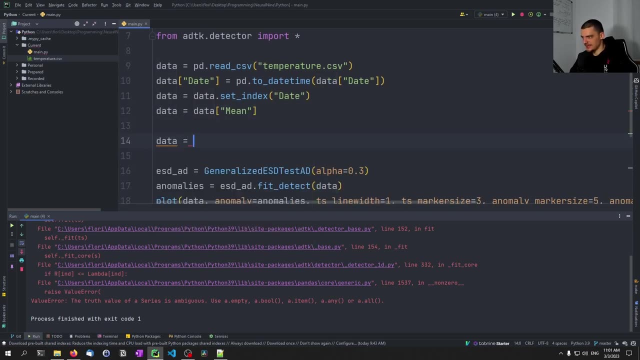 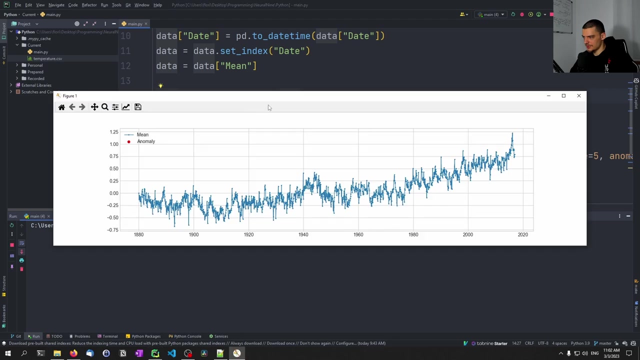 distributed, and if it's not, um, what's the problem here now? oh, i think i know what the problem could be. we didn't validate the data. so i think if we say data equals validate series data, this should solve the problem. there you go. okay, that was the issue. um, in this case, we don't find any anomalies. 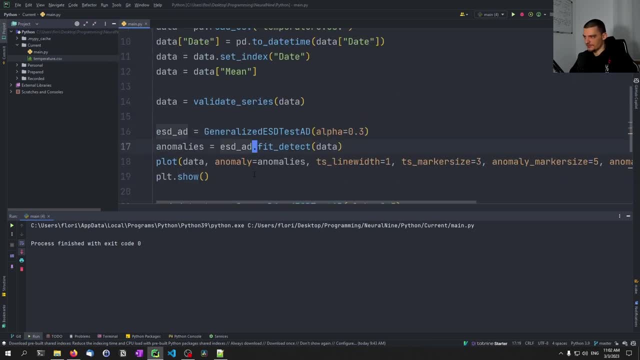 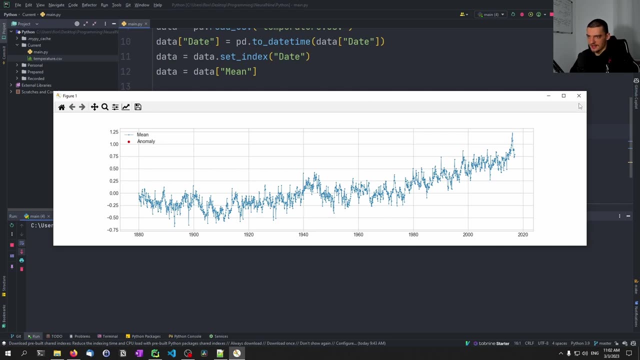 maybe it's because, um, we don't have any anomalies, we don't have any anomalies, we don't have any. uh, by the way, i duplicated the code here. let's run this again. uh, maybe it's because just the data is not normalized, maybe the alpha parameter needs to be adjusted, but since this data is not, 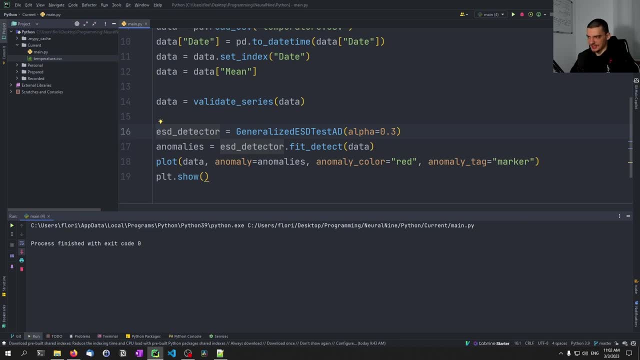 normally distributed. anyways, it doesn't make a lot of sense to use this detector here. i just wanted to show it to you guys. so if you have some data that is normally distributed, this might make sense. uh, to find anomaly detection. um, one thing that's very interesting, especially for stock. 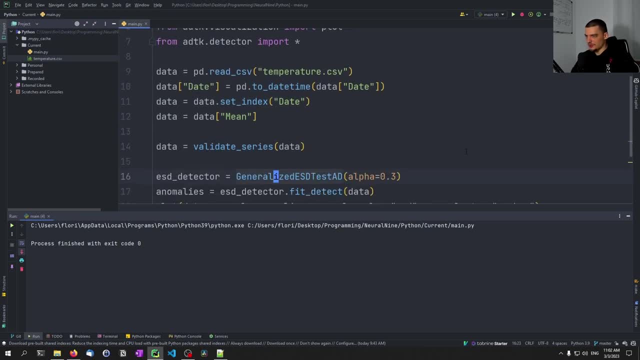 prices is the persist anomaly detection. so now we're going to proceed by using um, by using stock data. so i'm going to comment this out and we're going to say: data equals y finance. uh, actually, not y finance. yfdownload- we're going to download, for example, 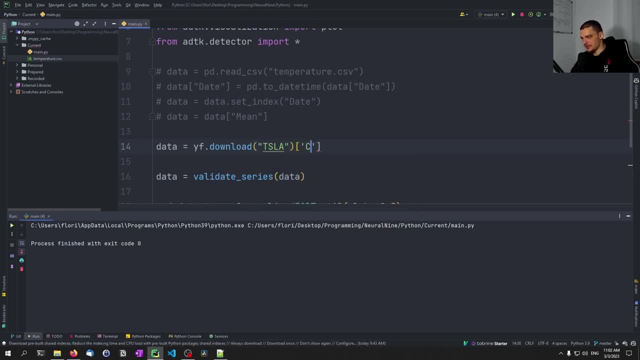 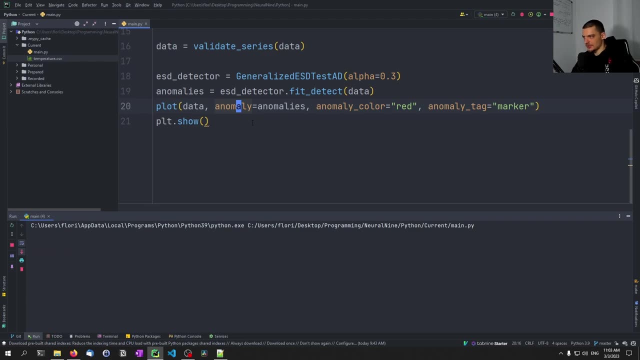 the tesla stock price and we're going to just pick the close column. we're going to then validate it. um, first of all, let's see if it works. there you go. so now we have the tesla stock price, uh, and this procedure is going to be used to validate the stock price. 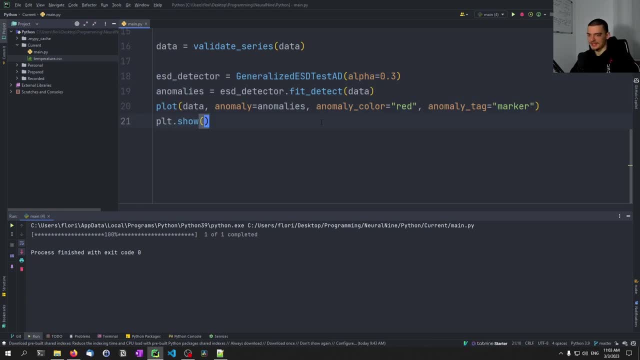 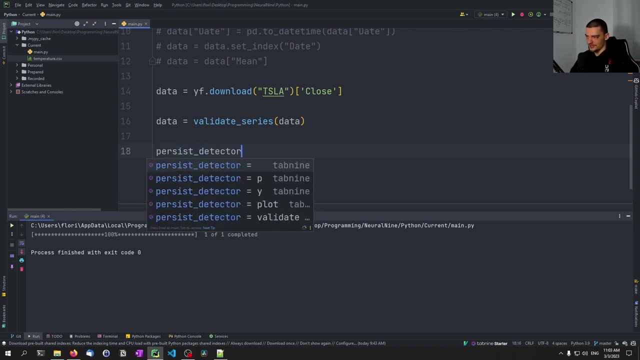 so we're going to say persist. uh, what is it called exactly this persist anomaly detection, basically. uh compares each value to the previous one and it detects positive or negative changes that are anormal. uh, that's the basic idea behind that. so we can say here, persist detector is going to be. 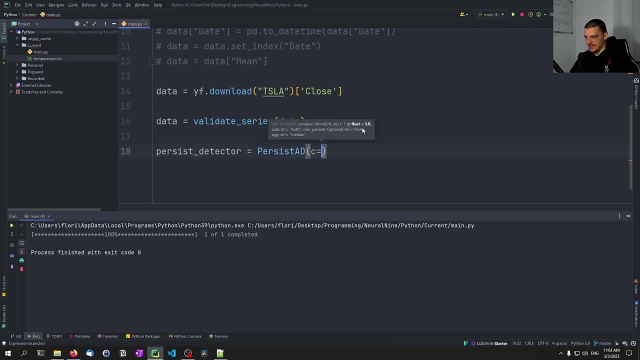 equal to persist ad. we can set again some tolerance here or some sensitivity 3.0, and we also just define here the site: are we interested in positive or negative sensitivity 3.0? and we also just define here the site: are we interested in positive or negative sensitivity 3.0? and we also just 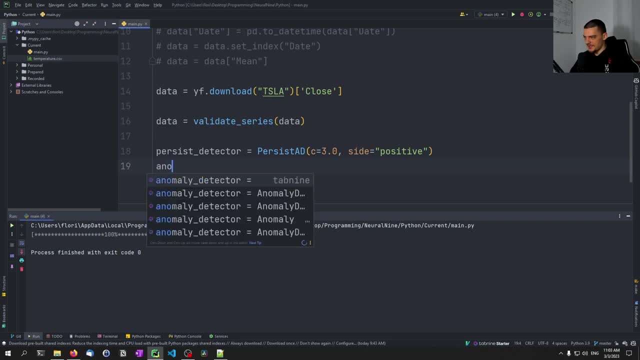 define here the site. are we interested in positive or negative sensitivity 3.0 and we also just negative movements that we want to detect um the anomalies again are: anomalies are computed by saying persist, detector, dot, fit, detect on the data and then we want to again plot the data, plot the. 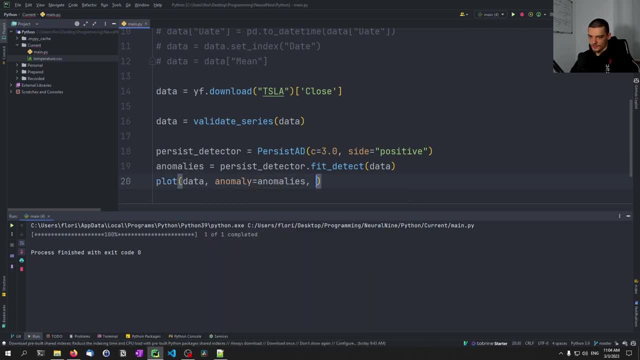 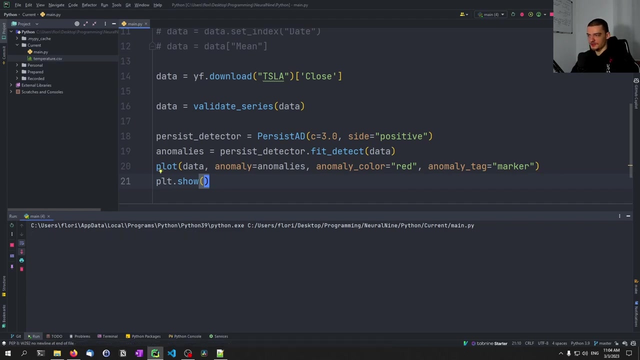 anomaly. we're going to then again say: anomaly, color red and anomaly. what did we have before? anomaly tag equals marker plt show. this basically shows us where we have some unusual positive price movements. in this case we have quite many. let's maybe adjust this parameter here to find less. 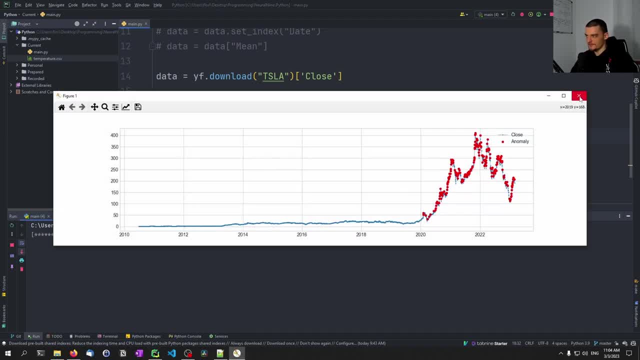 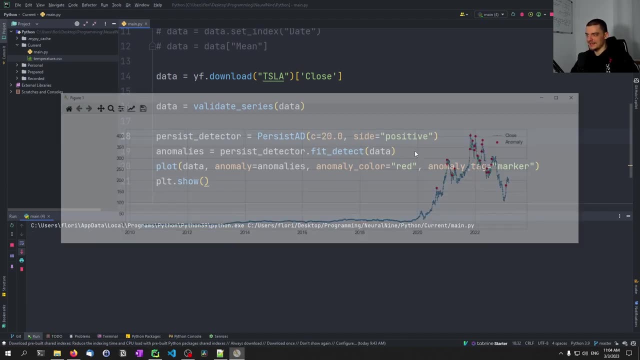 still finds a lot. maybe if i change this to 10- oh yeah, now it finds a little bit less. maybe let's change this to 20. let's see when we get only a few of them to get the essence. yeah, here you can see. maybe here we have a lot of price movement, here we have a lot of price movement. 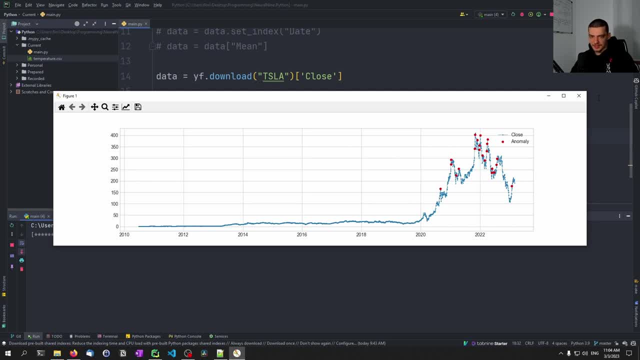 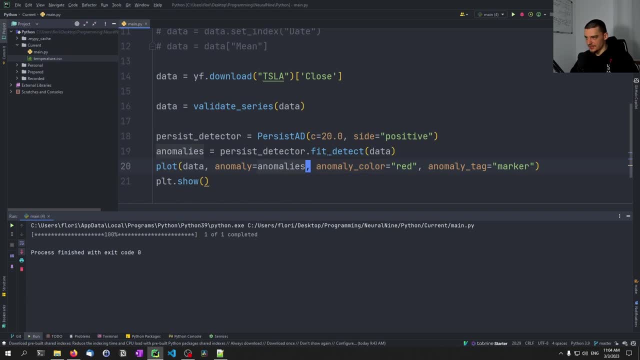 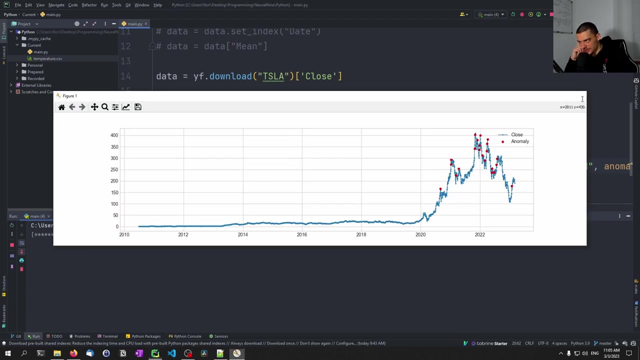 now for this one. actually it might make. uh, let me just see if we, if i can change the way this is plotted by saying: ts line width equals one, ts marker size equals three. maybe this changes the way this is displayed, because as far as i remember it was actually. let me just 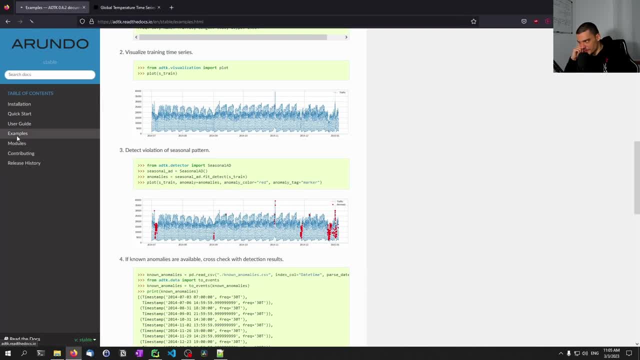 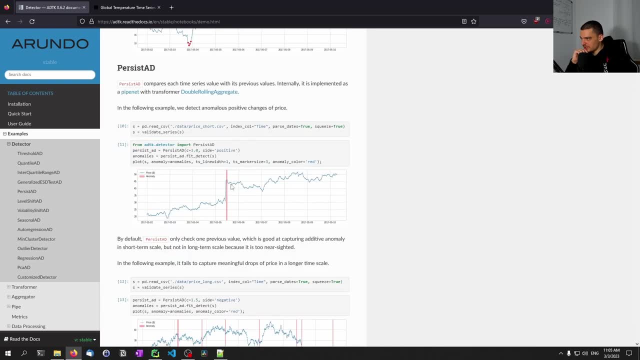 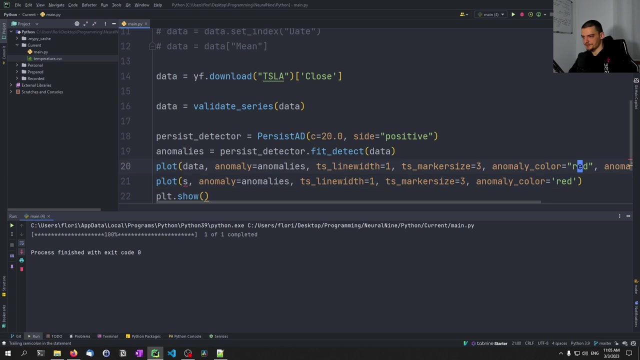 look up in a documentation. as far as i remember, when we go to the examples here, to the persist- yeah, actually it was displayed like this, so maybe we need to let me just copy this here: we do fit detect, we do the plotting, but i think actually i should have done this correctly, so i'm not sure if this is going to. 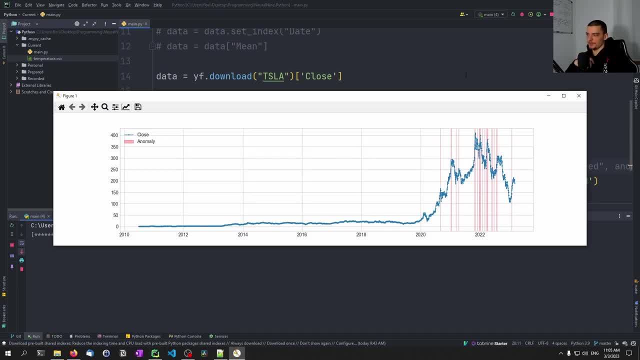 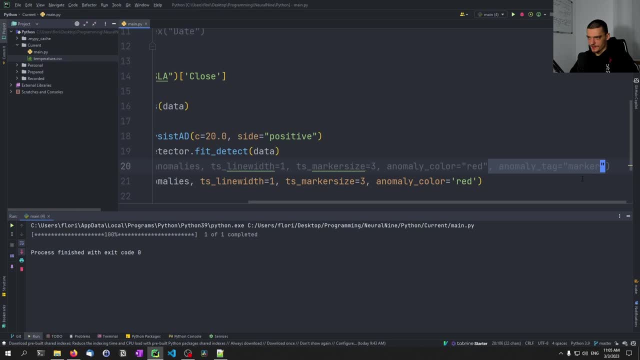 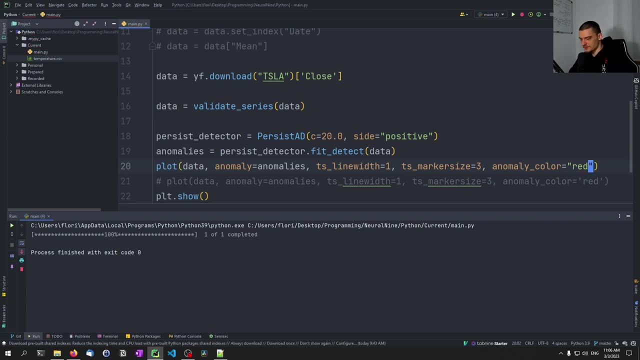 change much. there you go. now we get. what's the difference actually? let me just see that here. maybe it's because of the marker, maybe we shouldn't have the marker here. let me just see if that's difference should be a difference, i guess. yeah, there you go. so here you can see now where we have some anomalies. 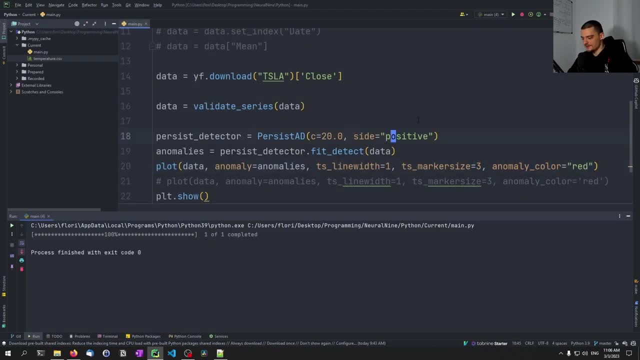 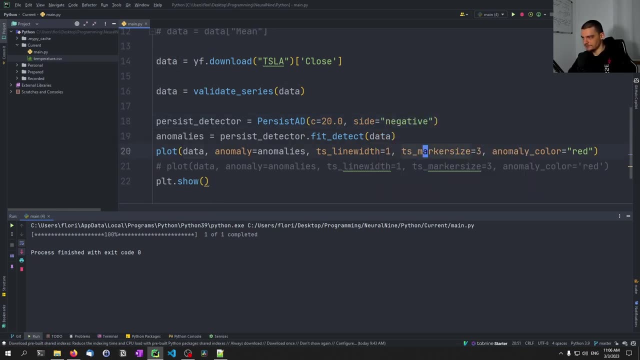 and same can be done for, uh, the negative side. so we can change this here to negative and then we can plot it again and this can be quite useful again, as i said, to spot some unusual movements. now it seems to detect way too much, so maybe we can adjust this parameter so that we find less and less. um, yeah, so here, for example, we can see: 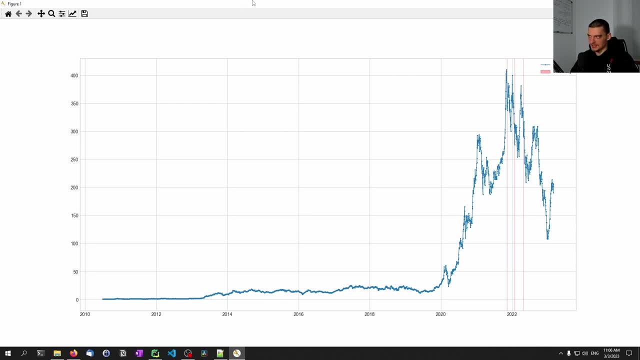 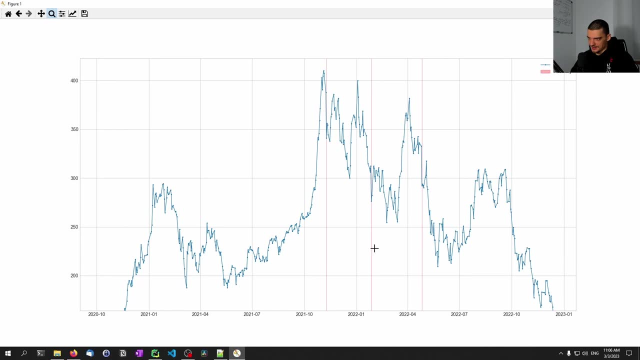 this is an unusual movement. this is an unusual movement. this is an unusual movement. maybe i can even zoom into those. there you go. so this is definitely unusual. uh, this is unusual. i would also say this is unusual. uh, but the thing is, it only recognizes- here um one day movements because 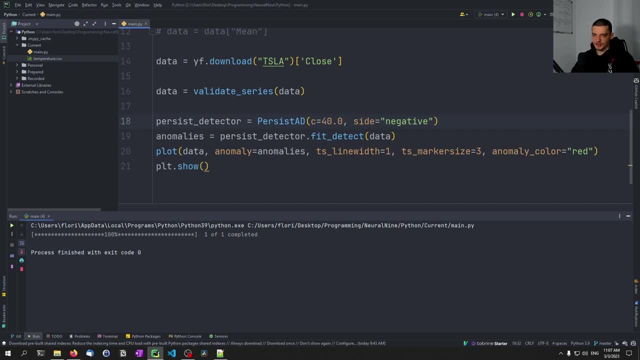 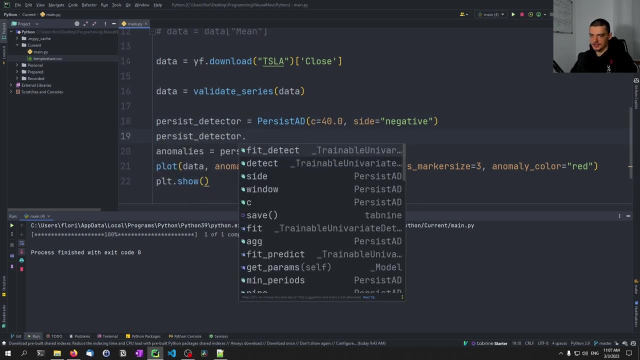 the window. the time window of this persist detector is one by default. we can change that by saying here: persist detector dot eight, uh dot dot window, sorry, equals. and then we can set 10 days, for example. then it's going to look back 10 days, um, and then we can see: uh, actually nothing. maybe we should be less sensitive here. 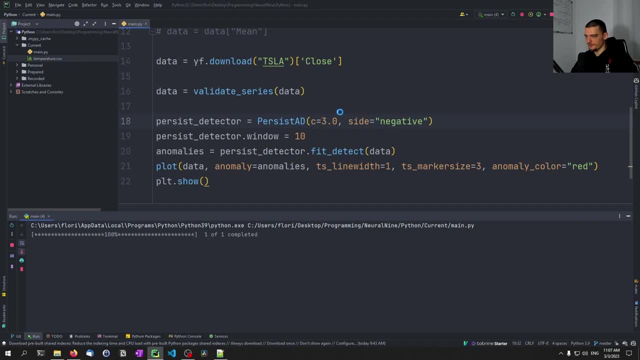 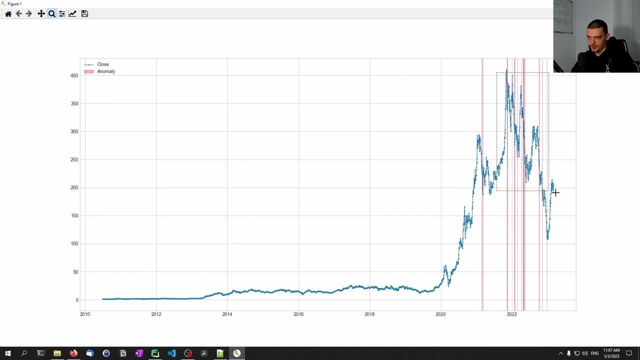 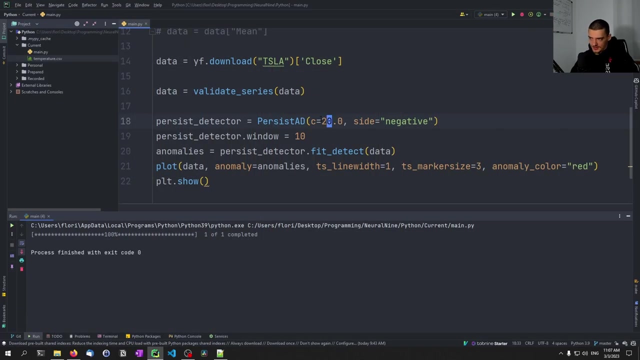 or more sensitive. sensitive here- okay, this is too sensitive. let me just change that here to 20. you can play around with that. right, you can intuitively see what makes sense and what not. let me zoom in here. yeah, i mean, we do get more results here. uh, you have to play around with that, but the basic idea. 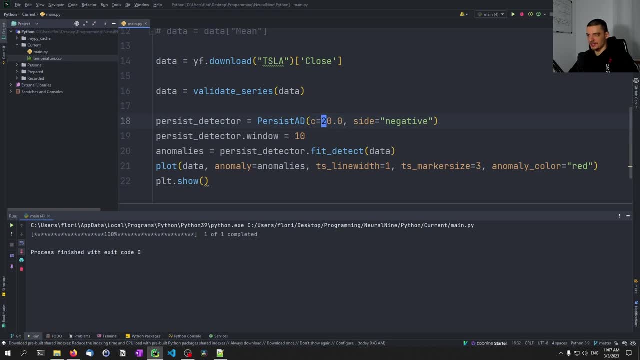 is you adjust the sensitivity here. the higher the number you set uh c to the less detection, the less anomalies you will detect, and the lower you set it, the more anomalies you will detect. and um for the window, you can adjust how many days to look back. that's the basic idea here. 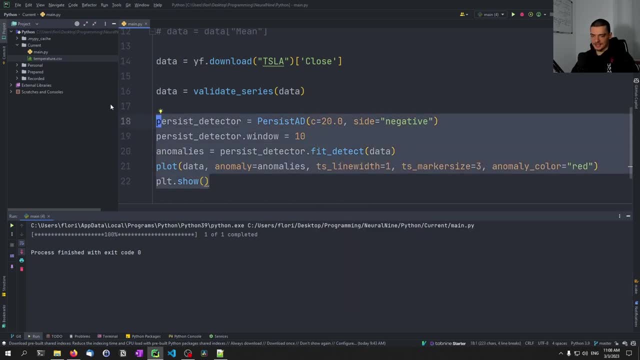 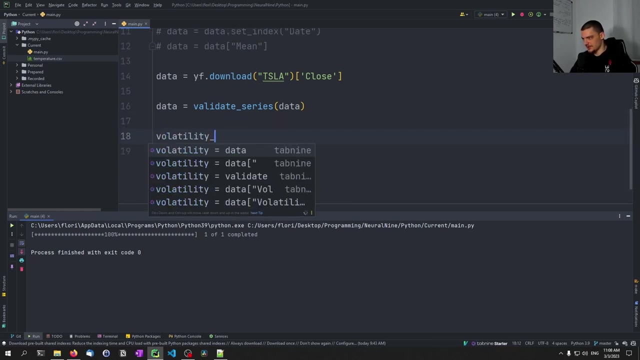 now, last but not least least, what I want to show you here is something that we probably won't see in the Tesla stock price, I guess. at least maybe we will. we can do some volatility detection here as well. so this is the volatility shift anomaly detection. we can just say volatility underscore detector. 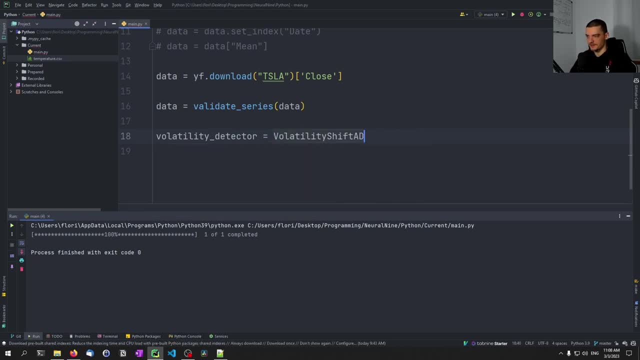 is equal to volatility. shift ad. we can set c to 6, we can set the side to positive and we can set the window to 30 instances. then the anomalies, anomalies are again going to be volatility detector, dot, fit, detect data, plot data. anomaly equals anomalies. anomaly color equals red and then we can say plt, show. 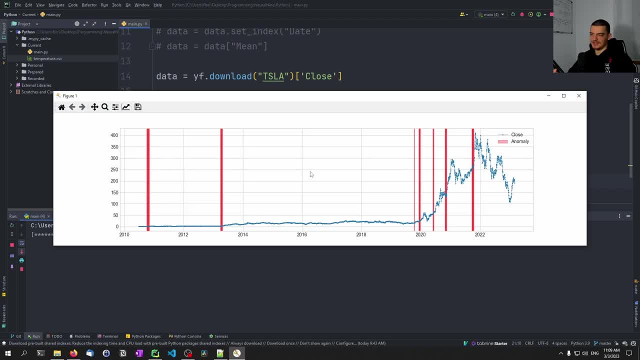 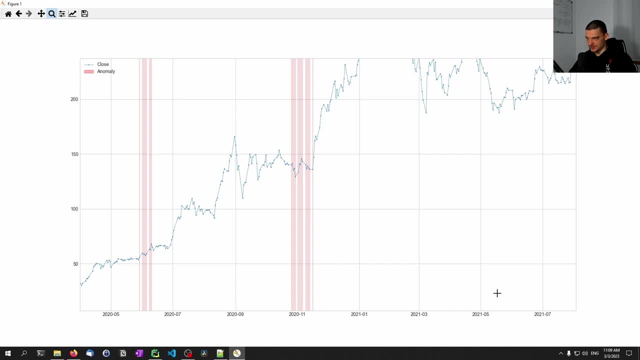 so the basic idea here is that we detect shifts in volatility. actually, we do get some results here, so let's see what happens here. let's maybe zoom into this here. it seems to be the case that at least the detector says so, that the volatility here seems to be a normal compared to what we